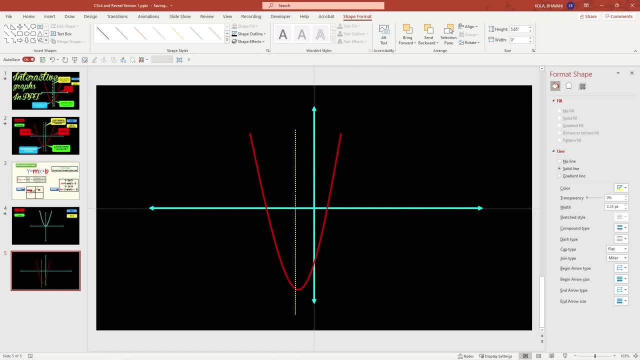 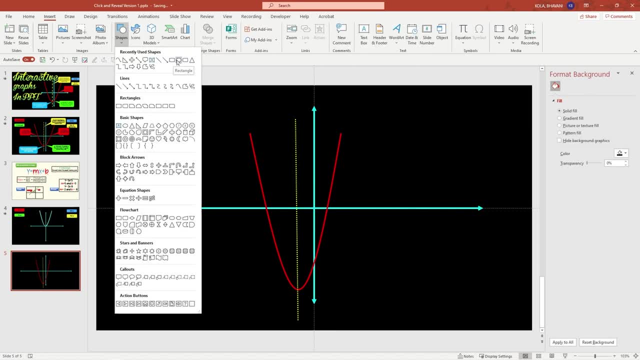 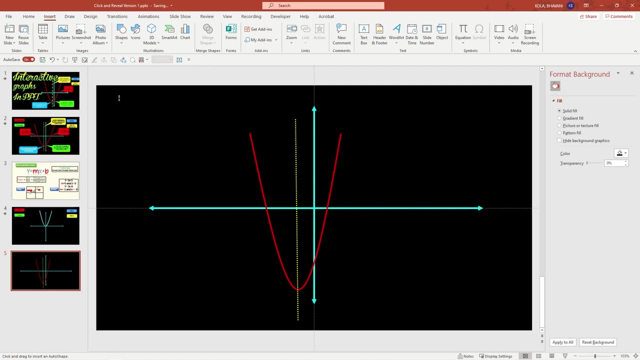 and change the type to dashed lines. And here is my axis of symmetry. I'm going to increase it just a little bit. The next thing I'm going to do is insert my buttons where my students click on them and the animations come to life. So the first one is for x, intercept, control and drag. 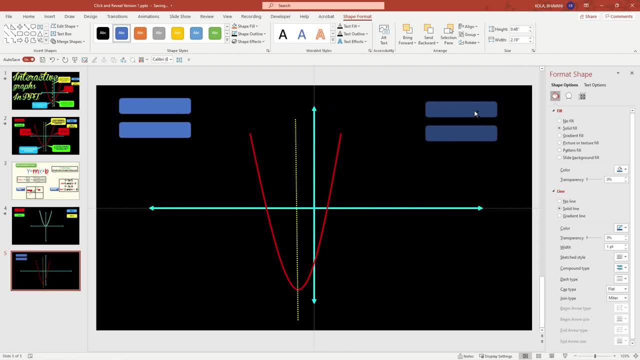 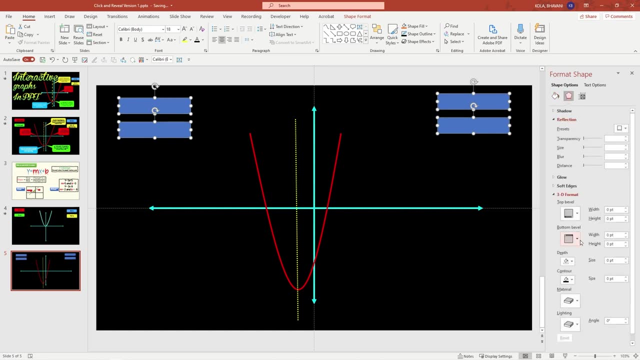 one is for axis of symmetry and other one is for the vertex. Once I have that, I'm going to select all of these. make sure I have no line In the shape options. I am going to give them a 3D effect. Once that is done, I'm going to insert shapes and I'm going to insert my callouts- Callouts. 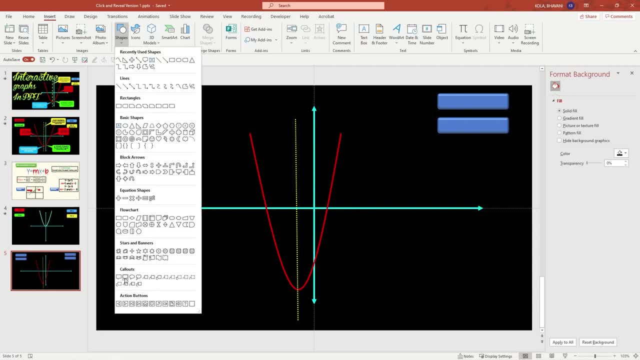 are the best way, instead of having to do it the whole time. I'm going to insert all my shape options, So I'm going to do that Now. make sure I'm going into the callouts tab. I'm going to insert my line. I'm going to put my line there in here. Make sure the line will stay in the shape options. I'm going to insert my line 1,2,3,4,4,5,5. 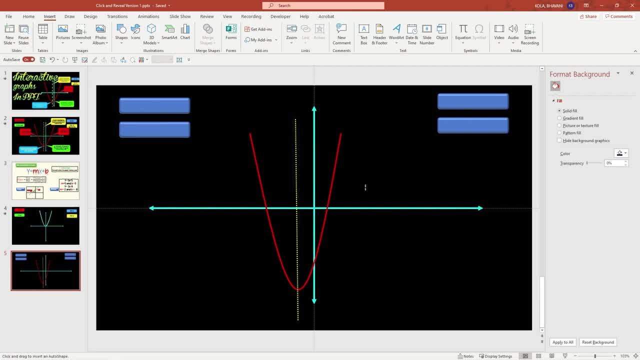 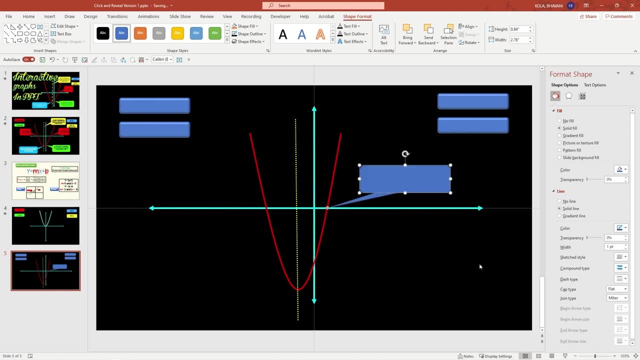 instead of having your text boxes and arrows. you're going to see why in a minute i need two call outs for my x and y intercepts. so my first call out is for my x intercept and, as you can see, this little yellow button, drag it and point it out to your x intercept. as simple. 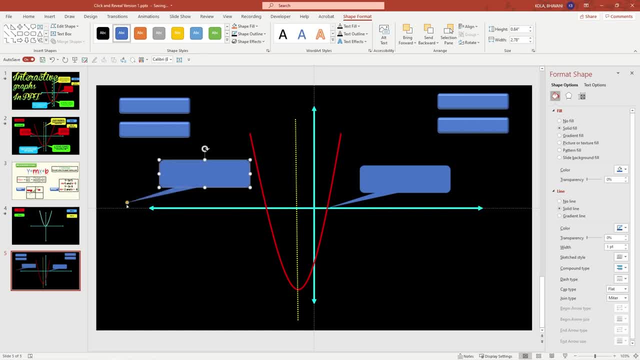 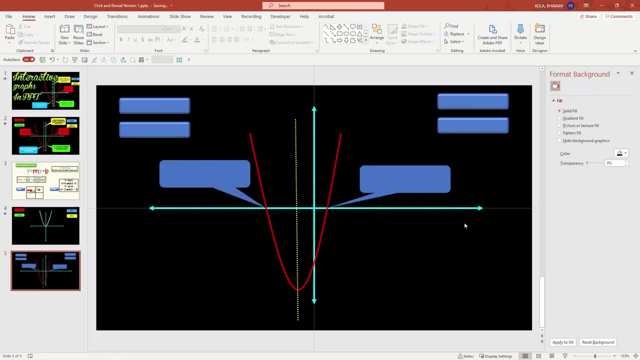 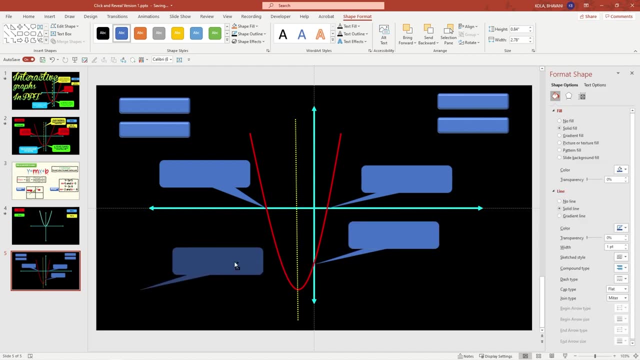 as that control. drag on the other side, move the yellow one to your x intercept and with one click you have a call out and pointing towards your x and y intercepts control, y intercept control and vertex control and axis of symmetry. again, i'm going to select all of these. 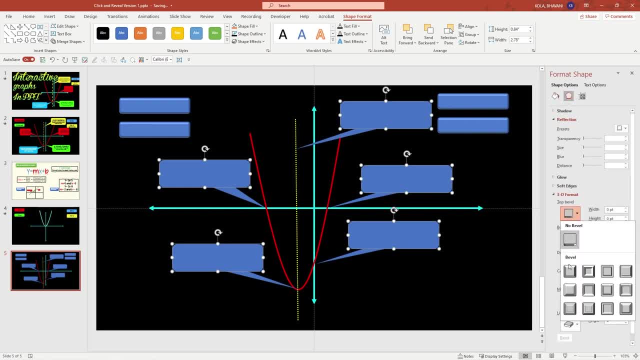 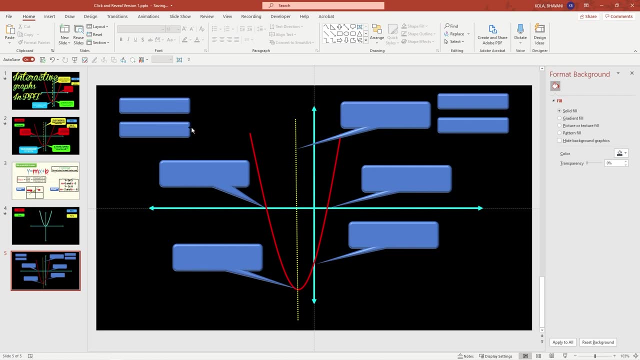 no line and i'm going to give them that 3d effect, shape options, shadow 3d format and pick whatever effect you want. now i want to make sure that my tabs and my call outs match the colors, so i'm going to go ahead and change all the colors. 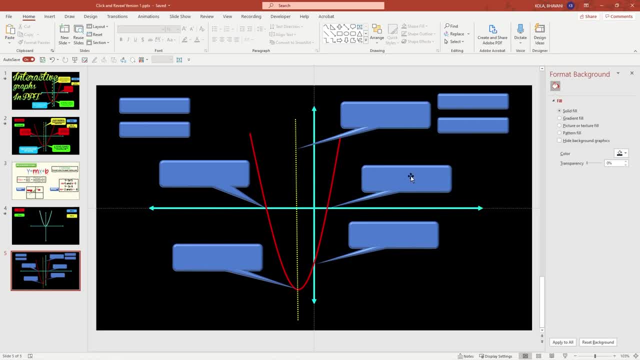 so these two are my x intercepts and i want them to be red. so select and change the color to red. i'm going to do the same for the rest of them and i'm going to be right back. all right, once this is done, let's go ahead and insert the x intercepts, y intercepts and the. 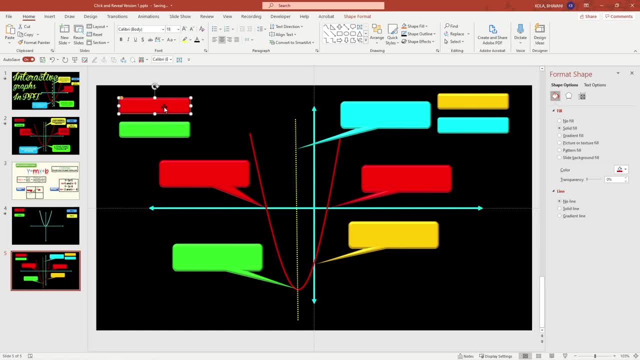 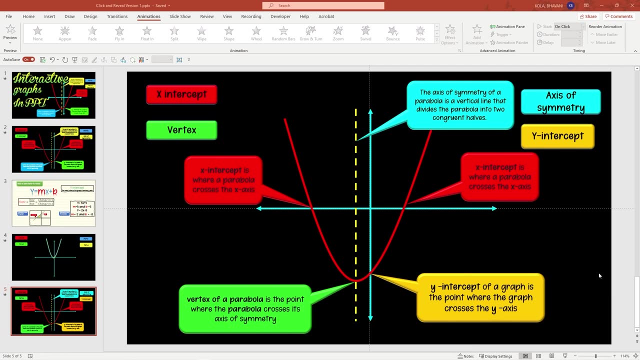 definition. all you have to do is double click and insert x intercept. let me go ahead and fill all of them and i'll be right back. so i went ahead and added the text to all my rectangular boxes and my callouts. now the next step is to bring this: 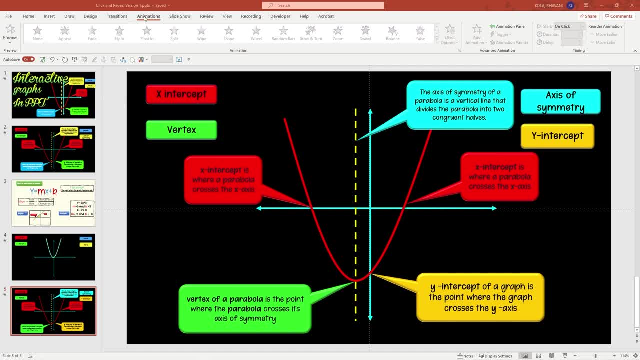 graph to life. so let's go ahead and add some animations. i'm going to click on animation, i'm going to click on my call out box and i want it to grow and turn. so please play with these animations and see what you like. This is the one that I like, so once I have decided what I want, 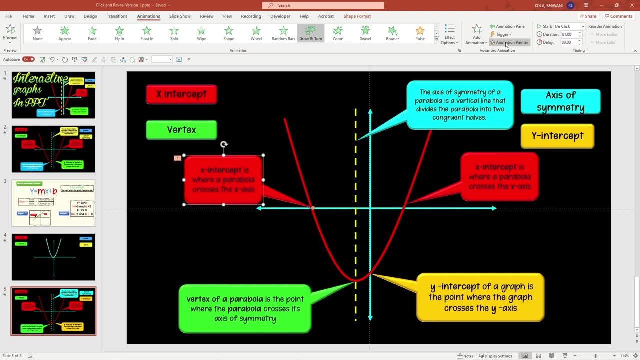 I'm going to click on the callout and I'm going to use my animation painter, So you will double click until you get the animation brush and, once that's done, go ahead copy the animation to all your callouts. All right, now that the animations have been copied, the next step is to add triggers. 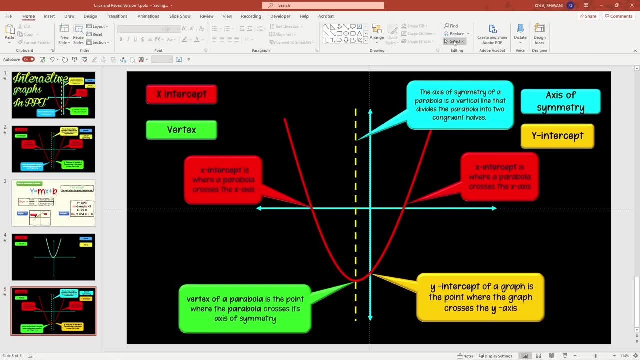 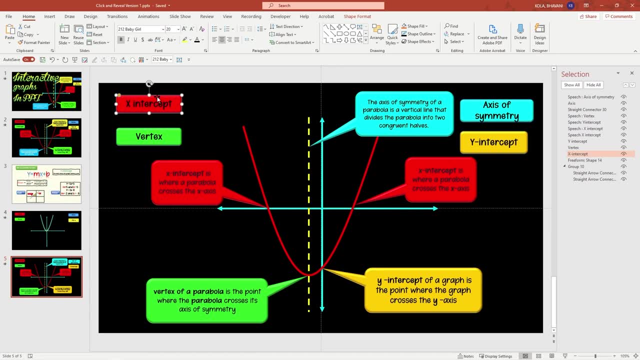 Before you add triggers, let's go to home, select selection pane and name these rectangle boxes just so that when you're adding your triggers it becomes much more easier for you to identify. So when I click on my x-intercept, as you can see, this has been highlighted. that's my x-intercept. 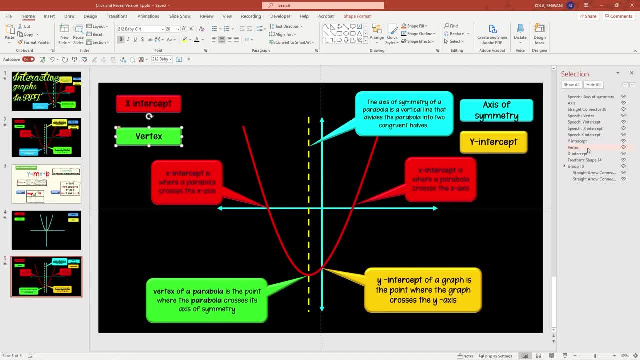 When I click on my vertex, it is the vertex. All you have to do is double click and type in the name that you want. I kept it same as the boxes, so when I click on my vertex, it is the same as the. when I'm adding triggers, it's easy for me to find out, So once I finish adding the names to all four. 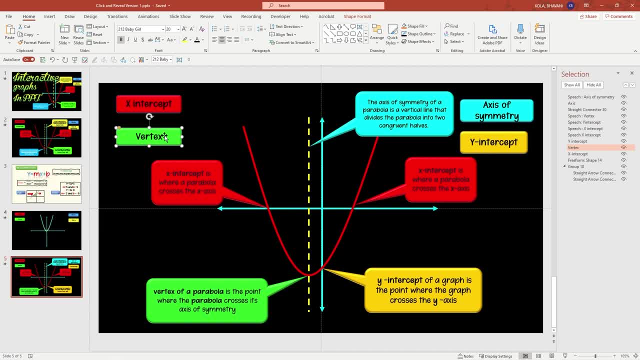 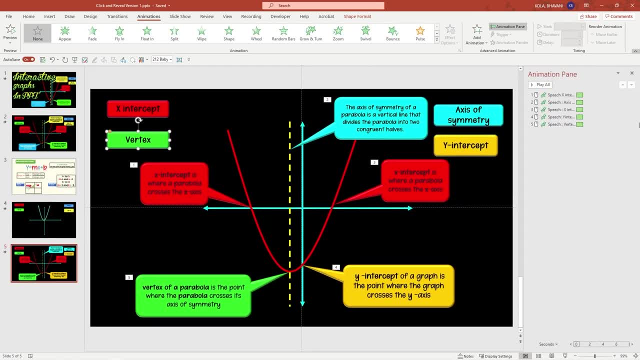 of my rectangular boxes. now it's time to go ahead and add those triggers. I'm going to close the selection pane, go back to animation, animation pane and I will start with my y-intercept callout. So I'm going to click on my y-intercept and I want this animation to come to life only when I click. 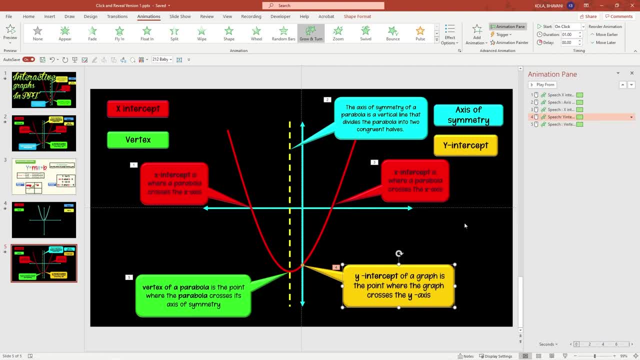 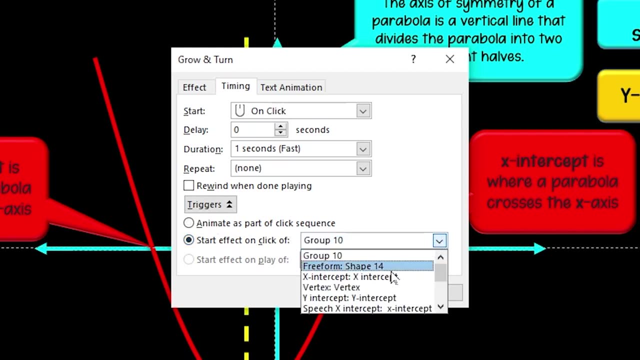 on my y-intercept rectangular box. So once I click on it, as you can see, it's going to come to life. As you can see, this has been highlighted. I'm going all the way to this arrow: click on timings triggers, start effect on click of. go all the way down until you find your y-intercept. Now let's go. 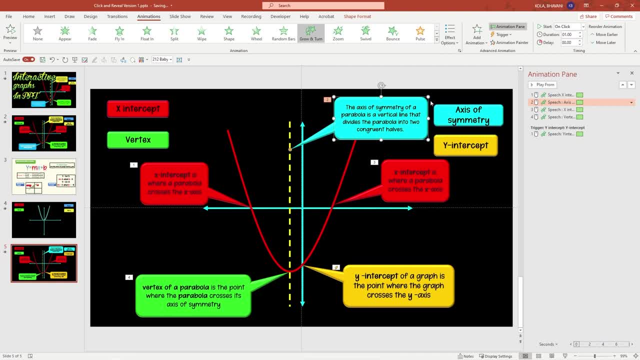 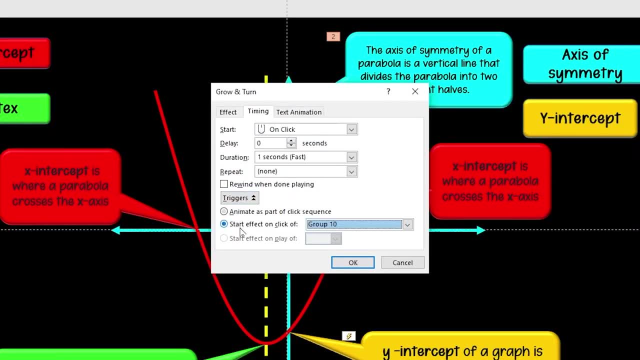 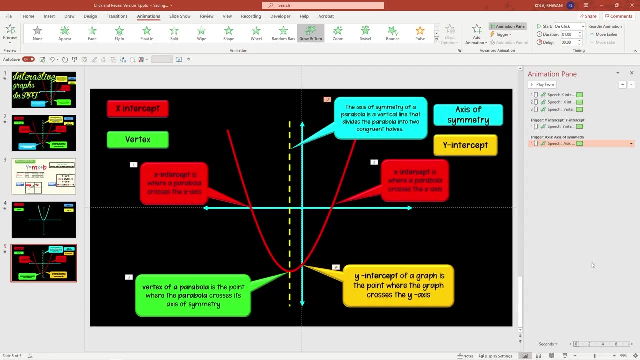 ahead and check for axis of symmetry. So when I click on my axis of symmetry callout, as you can see, it has been highlighted. The same procedure again: timings, trigger, select, start effect on axis of symmetry. Where is it? I'm going to go ahead and do the rest for all the rest of the 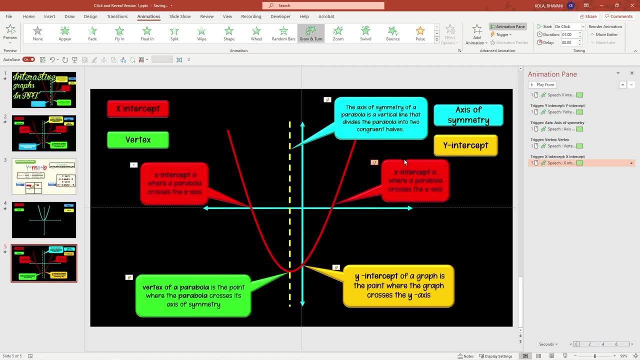 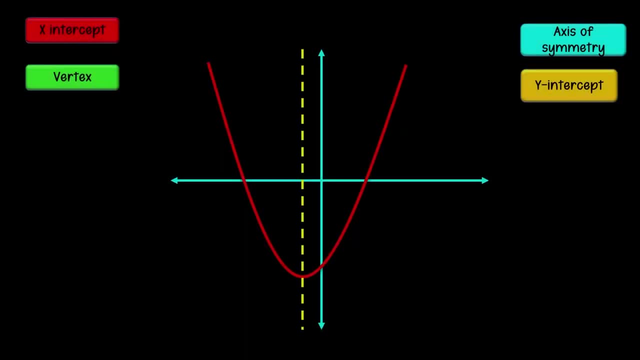 callouts. As I have two x-intercepts, all I have to do is add a trigger for the first x-intercept and drag the next one below it and make sure it plays with the previous. Now, once all the triggers and animations are done, let's go ahead and check this out. All right, x-intercept boom. 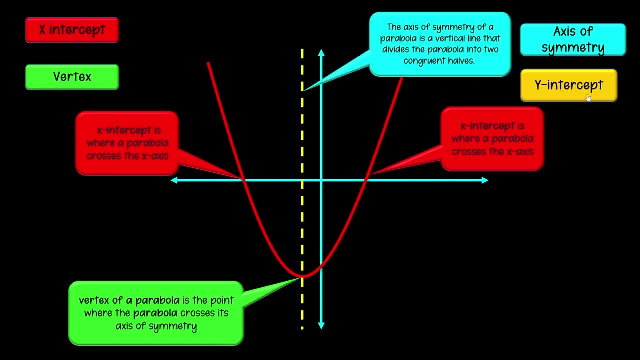 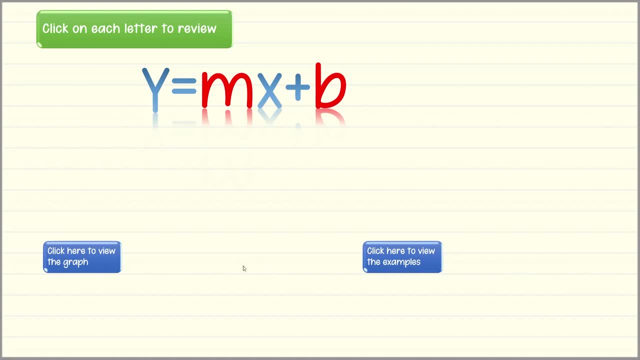 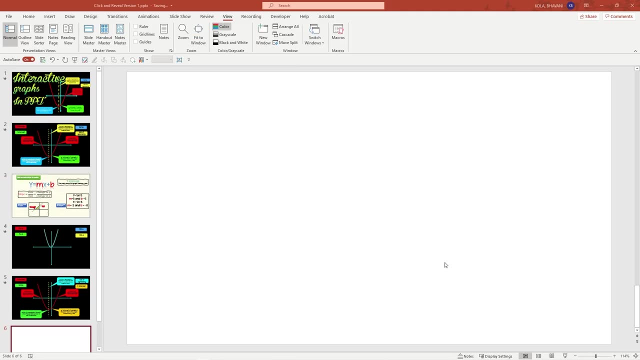 Vertex boom, Axis of symmetry, perfect, Y-intercept- perfect. Now that we have seen how to create interactive graphs, let's go ahead and take a look on how to create these simple math lessons with examples and graphs. So here I am on a blank presentation again, Right click format background. I want to 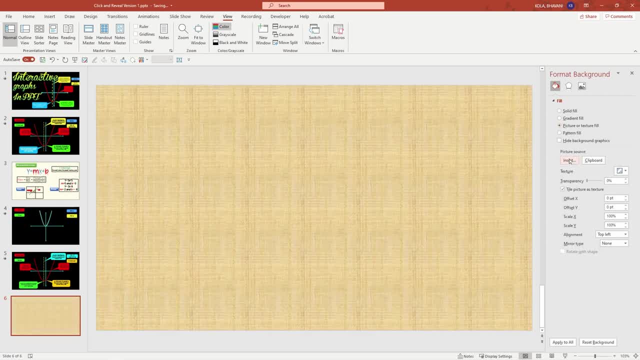 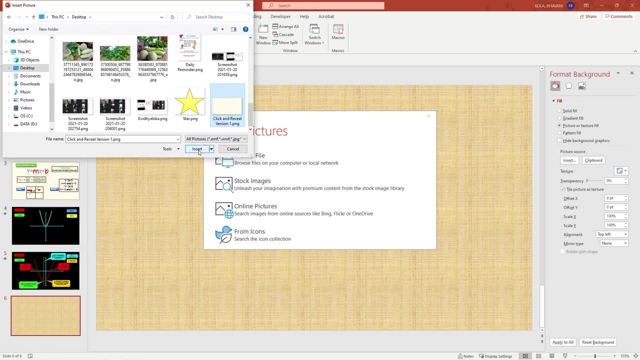 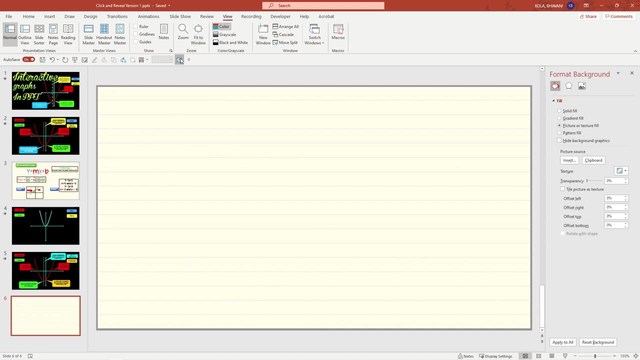 give it that notebook effect. so I'm going to click on picture and texture. insert from the file- I saved it on my desktop- Select the one that I want and insert. Once this is done, I'm going to go ahead and add text boxes. 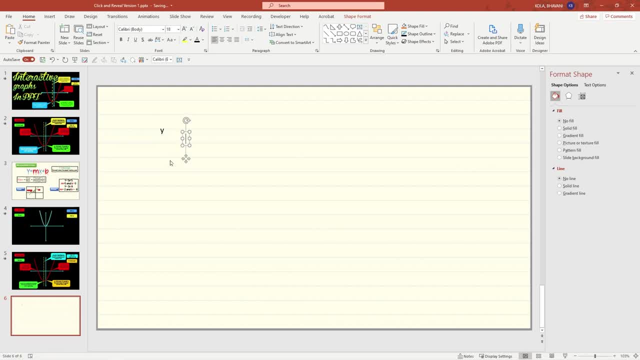 for each letter. So one is for y, one is for equal to one for m, one for x plus nb. You get the idea. Once this is done, I'm going to select all of these and make sure I align them to the top. 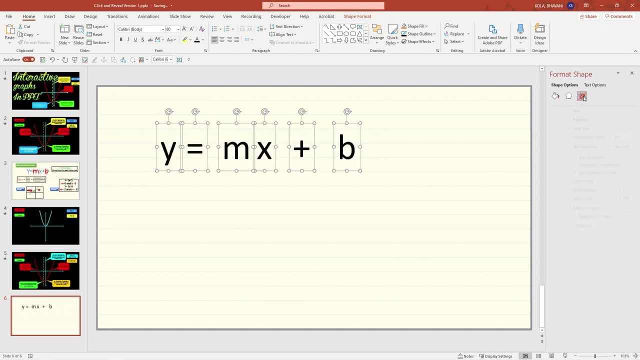 Increase the width. This is good enough. Click on my text options And I'm going to add it a shadow. So I'm going to click on the reflection and pick the shadow that I want. I think I like that. That's good enough. Change the font and I'm going to move this all. 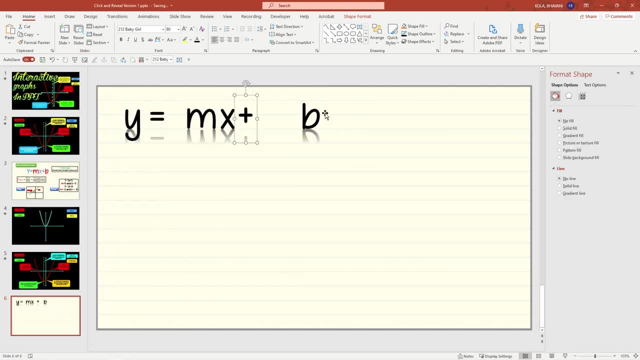 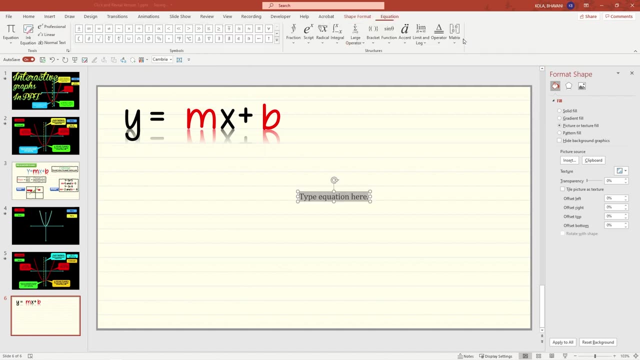 the way to the top here, and I'm just going to arrange them one next to the other. I want to change the color of m to bright red and the color of b as well. Now, once this is done, I want to go ahead and add the formula for the slope, So I'm going to click on insert equation. 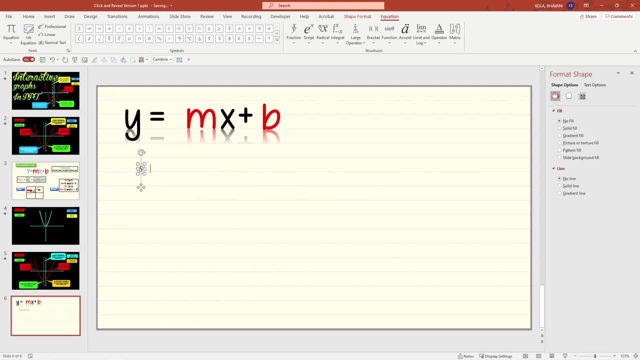 and here I have a brand new equation. I'm going to say: slope equal to. I want it in the format of a fraction. So I'm going to click on fraction and pick the style that I want. I think I want this one. I'm going to say slope is rise over run, which is nothing but change in y, change in x. 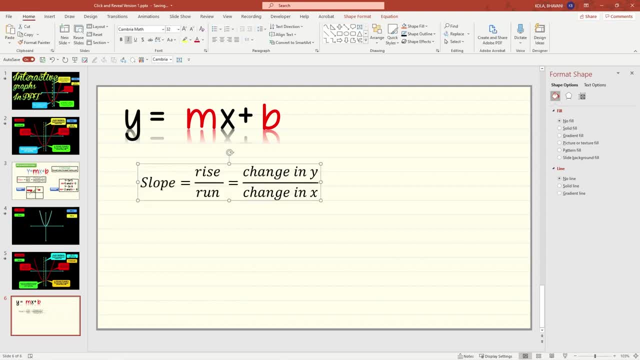 Once this is done home, I'm going to increase the size. I'm going to add an outline, Increase the weight of the outline and give it that sketched look. That's perfect. I'm going to add another text box and say y intercept, Y intercept is the point. 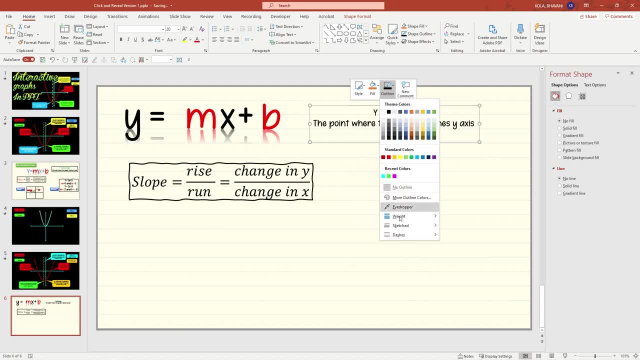 where the graph touches y-axis. Once that's done again, I'm going to give it the same effect and the sketched look. So right click on your text box- outline sketched, and there I have it. I also want to go ahead and add an example. I'm simply going to copy: 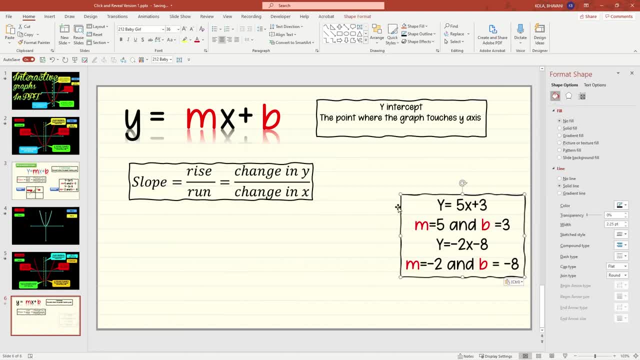 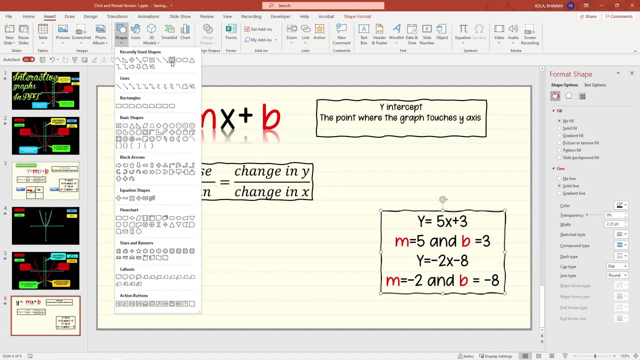 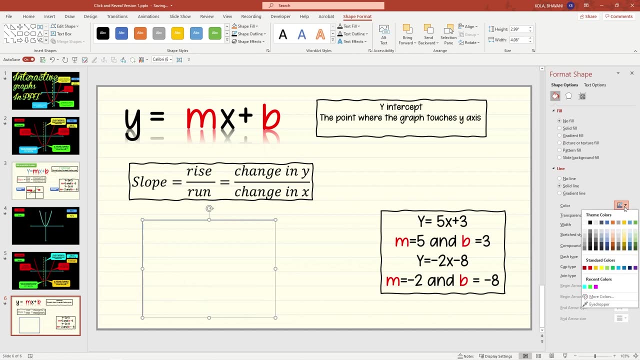 it from this one. So here I'm adding an example, and now I want to go ahead and add a graph. So I'm going to create a graph. To do that, I'm going to click insert a rectangle. I do not want to fill this with anything, but I want the line to be nice and black and I want. 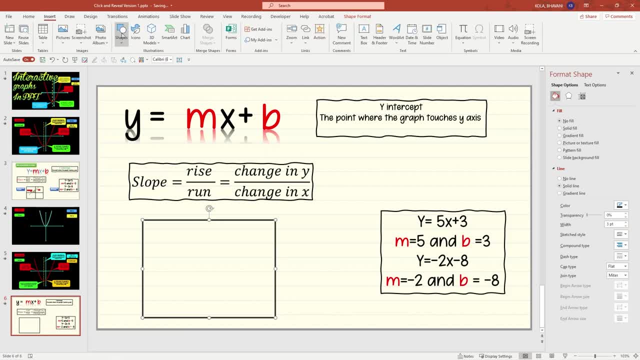 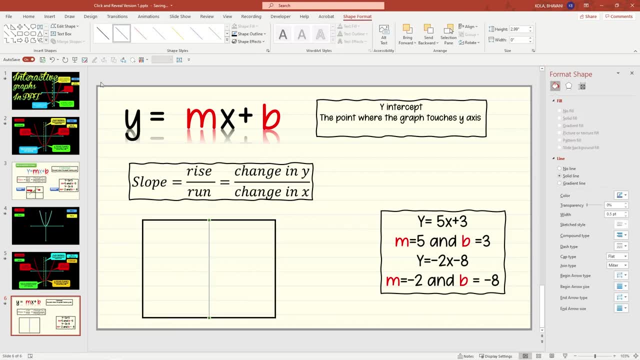 to change the width of it. Once that's done, I'm going to insert my x and y and I'm going to add a line. So I'm going to select both of these and increase the width. I'm going to select all of this. 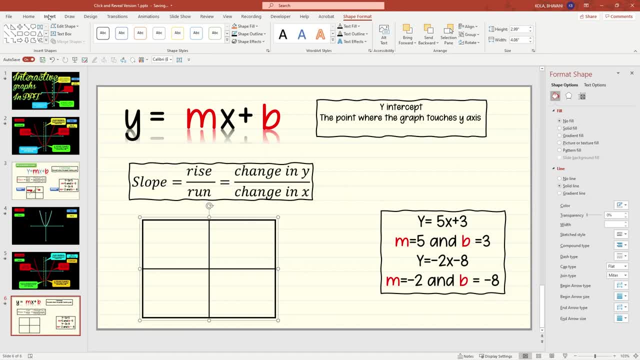 and I'm going to group it- ctrl g. And now I'm going to insert a line. Press and hold your shift button and increase the width. I'm going to select all of this and I'm going to group it- ctrl g. 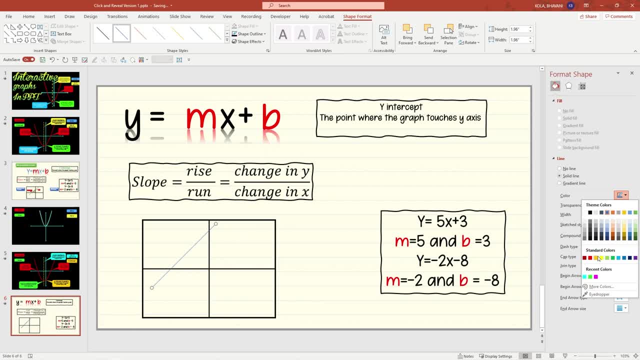 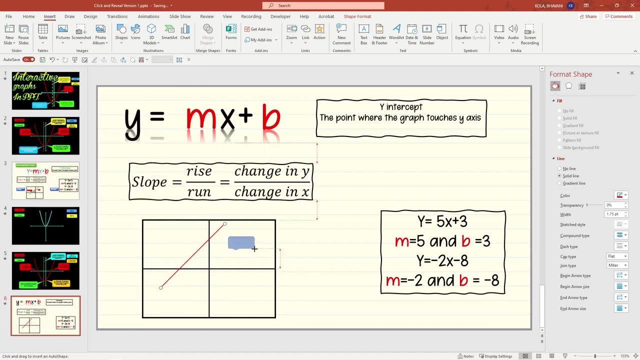 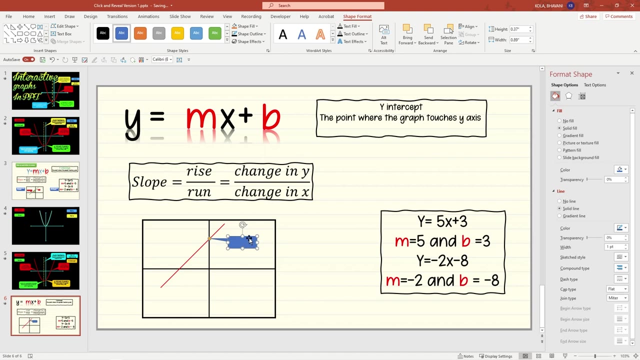 There is your line. Change the color of it so students understand it's a line that you're trying to focus on. That's perfect. Now I want to insert a call out just to mention my y-intercept and my x-intercept. So there is my y-intercept. Call outs are so much easier to do than a. 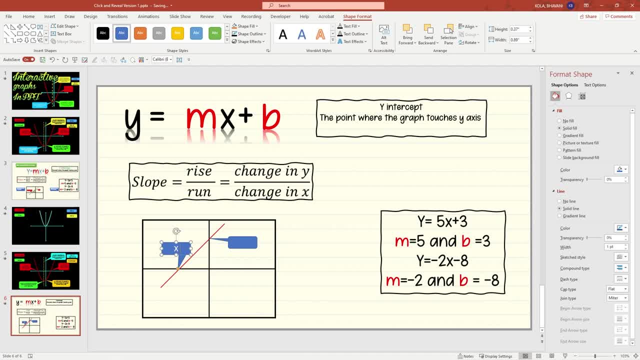 call out. So I'm simply going to double click and say x-intercept and this is b, which is my y-intercept. Make sure your call outs point out to the right direction. There you go, Perfect. And once this is done, the next step is to go ahead and add those buttons. 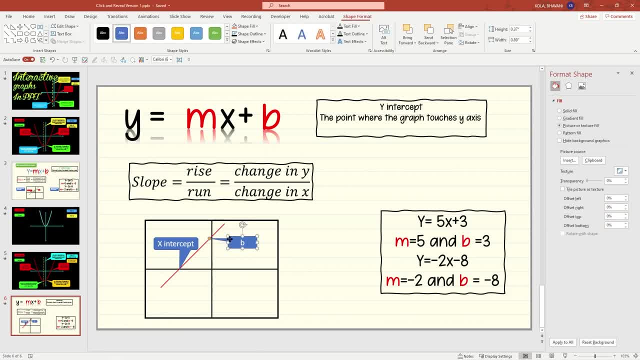 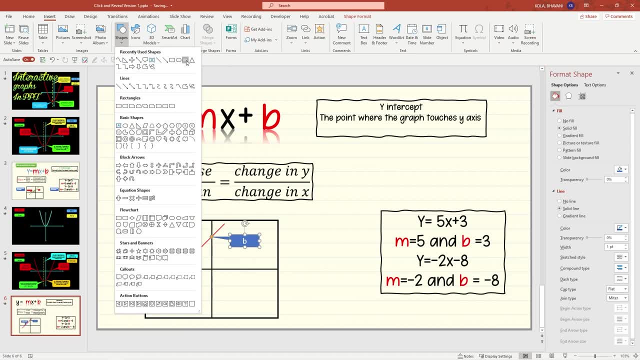 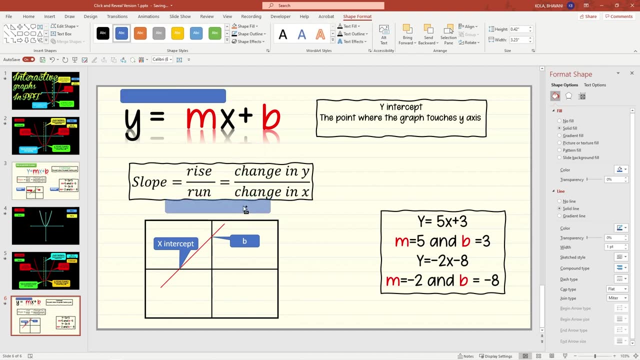 When my students click on it, the graphs and the examples and the formulas come to life. So to do that, I'm going to click insert shape rounded corner. So this is going to be my first button here: Control and drag it all the way down. Control and drag it all the way up here. 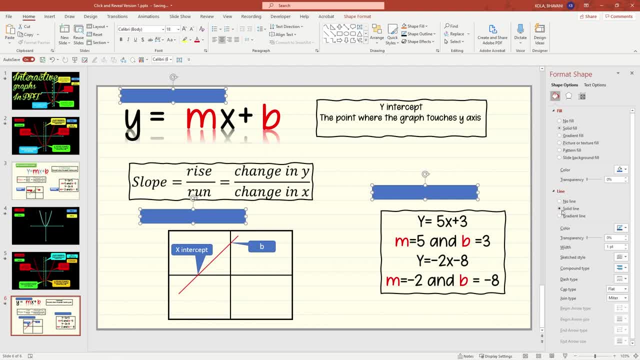 I'm going to select my rectangular boxes, no line. I'm going to change the color to green and I'm going to give it that 3D effect. like always, I'm going to go ahead and add some text. Alright, once all of this is done, 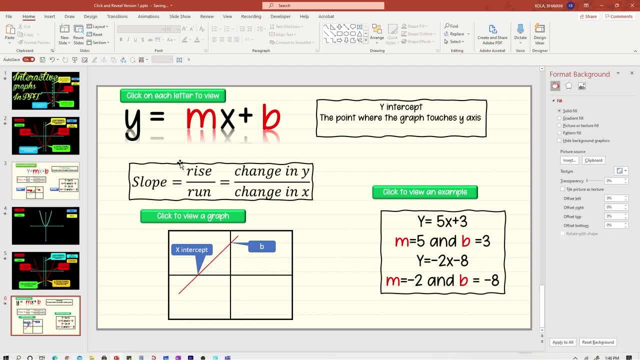 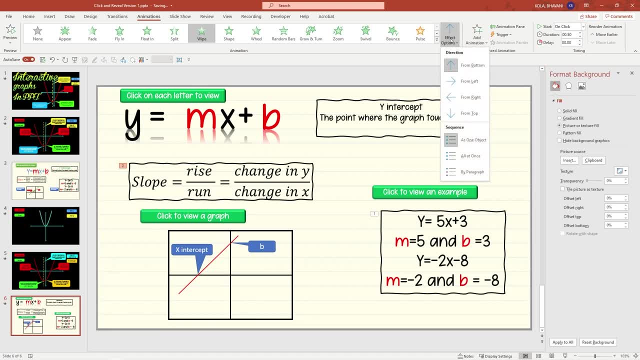 The next step is to go ahead and animate each one of these. So I'm going to click on my text box here- animation- and I want it to wipe- Not wiped from the bottom, but I'm going to make sure I click and say wipe from the left. 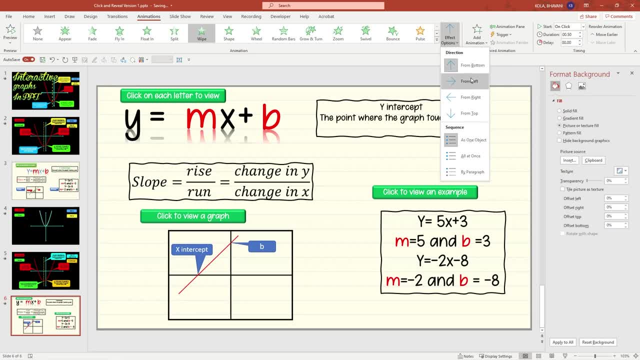 Go back here again. I want it to wipe Again. wipe from left. there I have it, The graph as well. I want to make sure I click wipe from the right or the left. This is going to point the end of the line. 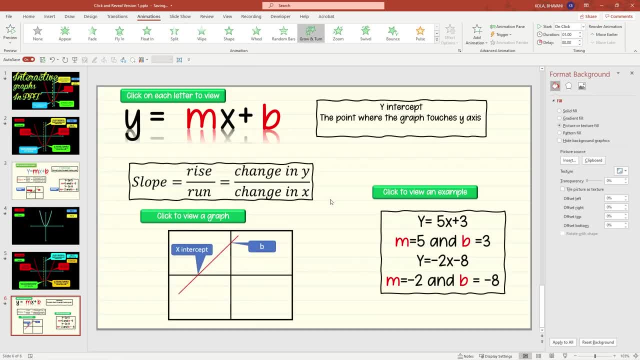 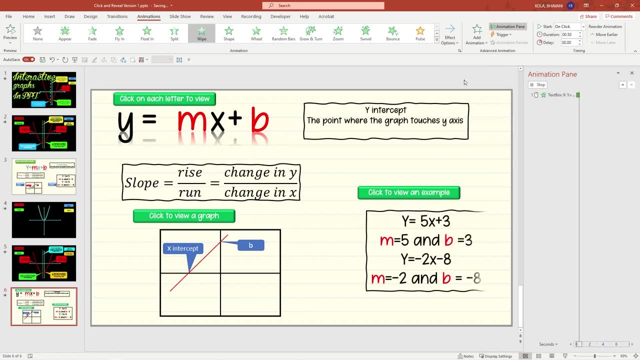 sure, yeah, i want the graph to come up something like that: perfect. so even this text example, i want it to wipe. i want it to wipe from the left, but i don't want it to wipe as an object. so i'm going to click on this little arrow timing text animation and i want it to wipe as paragraph. 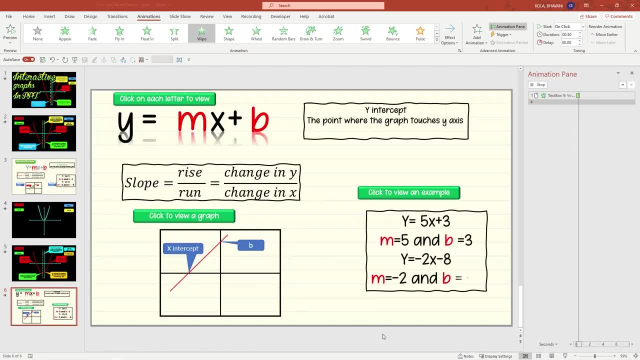 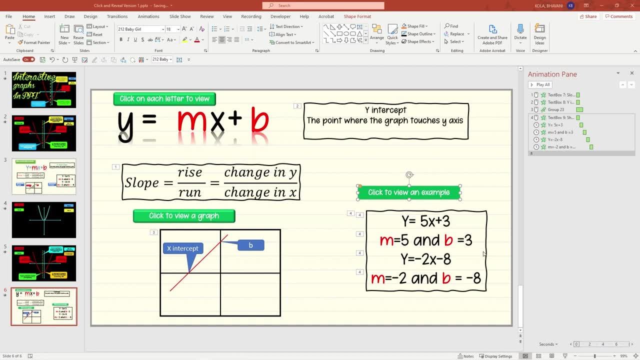 and let's see what happens. that's exactly how i want it perfect. so once the animations are done, the next step is to make sure we create and use those triggers to do that. again, i want to make sure you understand that you have to name these rectangles so you know exactly what they are. 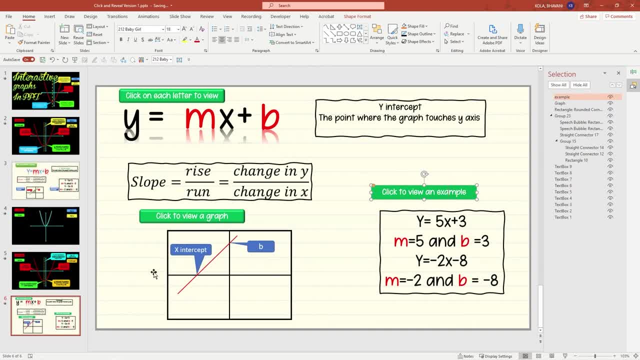 to do that, click on your home select selection pane, click on the rectangle- and i know this is the rectangle where i have my graph and this rectangle is where my students click and the example pops out. so that's an example to me. it's always nice to name your rectangles because when 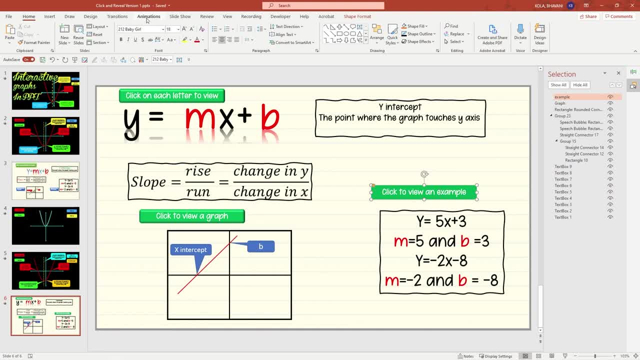 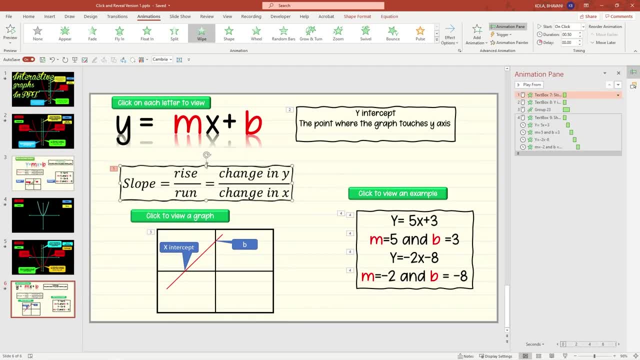 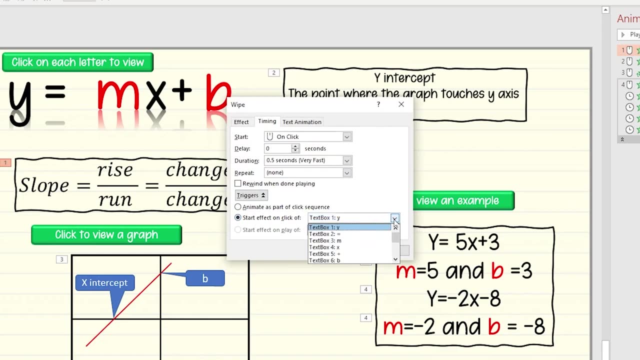 you're adding triggers. it makes your life much more easier. so let's click on animation, animation pane and i want the slope is equal to rise, overrun, to pop up when i click on, so start effect when i click on the letter m. so there you go. i just added my trigger. 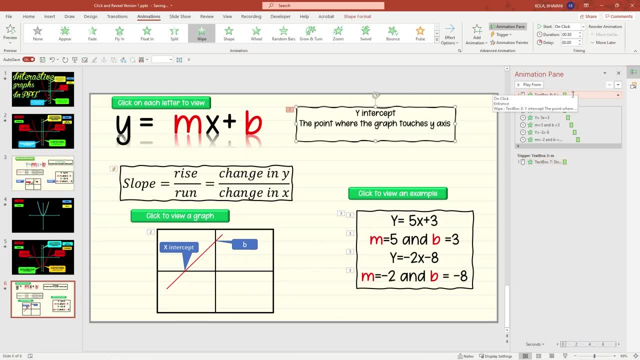 now i'm going to click on my text box here and this has been highlighted: timing triggers start the effect on and i want this to animate when my students click on the letter b. so now you know why i had different text boxes for each letters. this is my graph and i want the graph to animate when my students click on. 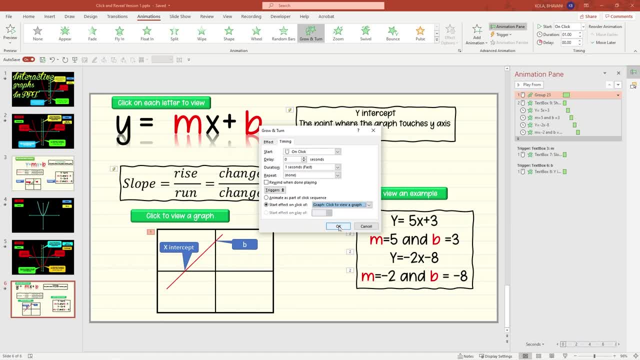 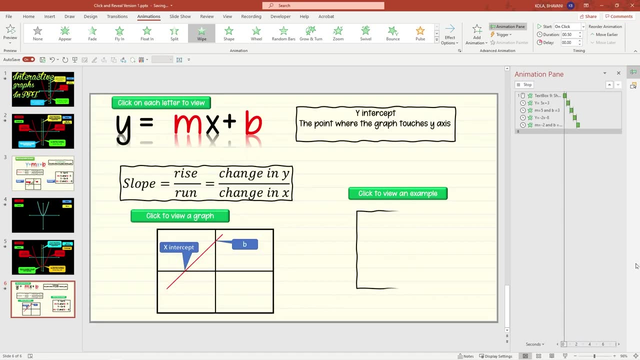 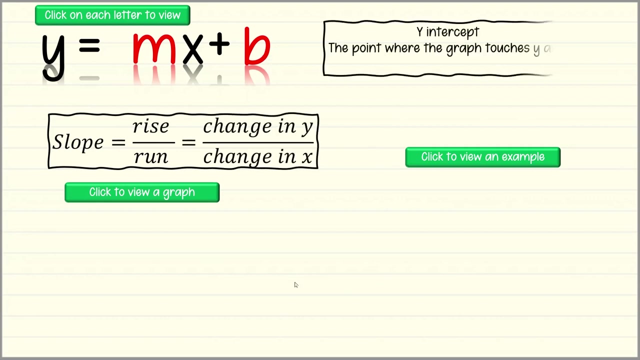 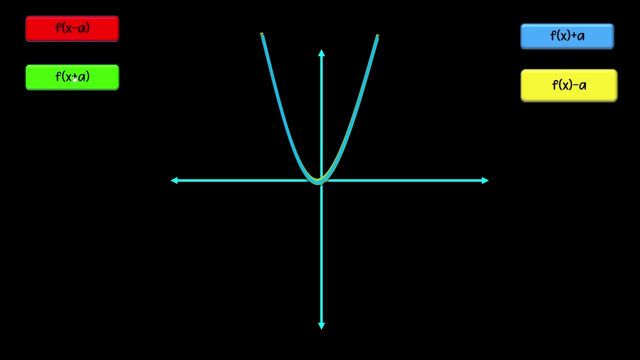 the tab or the rectangular box that says graph perfect and i want this to animate when my students click on view an example tab. so i want the graph to animate when my students click on the tab. now let's go ahead and test this out. so m b example and graph perfect. another variation of this could be transformation of graphs, where 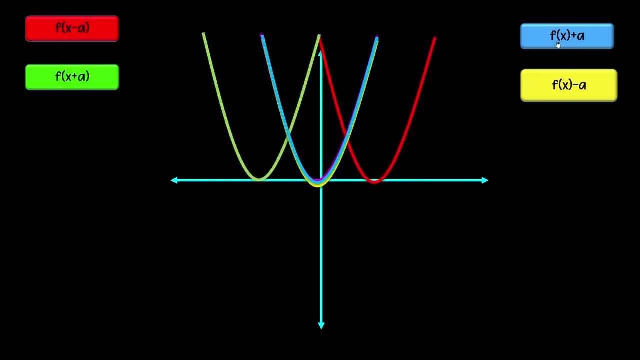 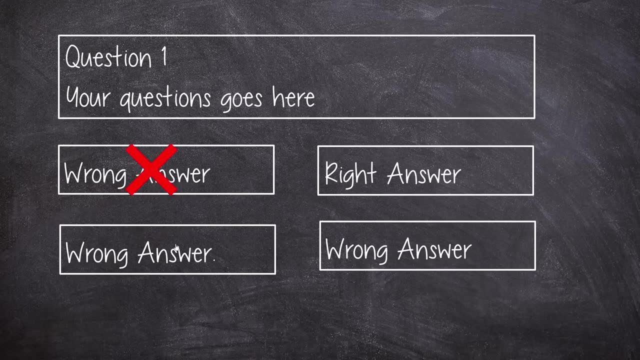 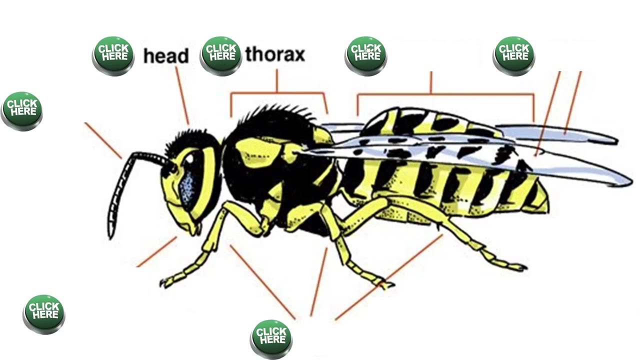 all the transformations are animated and coming to life. please stay tuned for many more interactive tutorials with powerpoint, like self creating quiz, click and reveal animated syllabus, and and much, much more. Would love to hear your feedback, so please leave a comment below and let me know what would you like to see more in my videos? 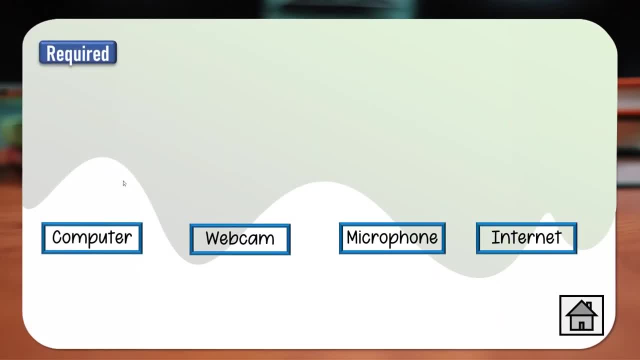 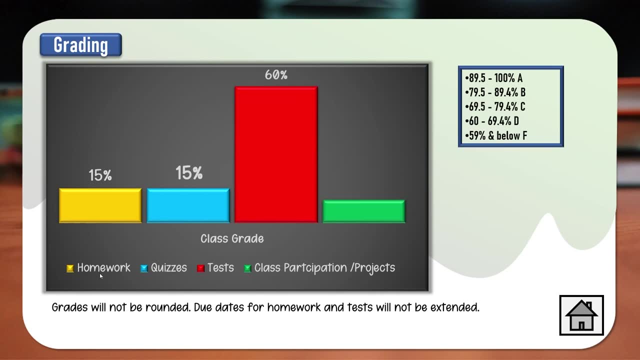 what worked and what did not. I hope you learned something new today. I hope you enjoyed the video. If you did, please make sure you like subscribe, and if you think it's worth sharing, please go ahead and do so. There could be an educator who might really need. 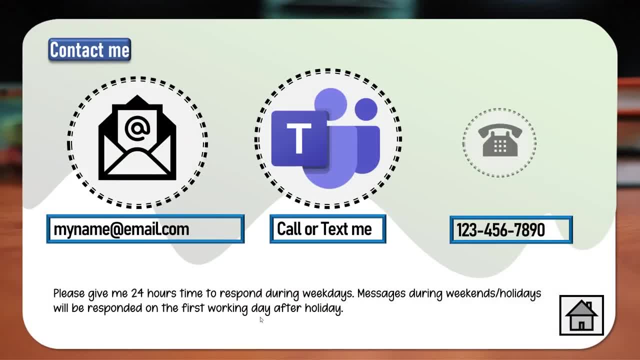 these animations for their classes And always remember: happy teaching and please take care of yourself.